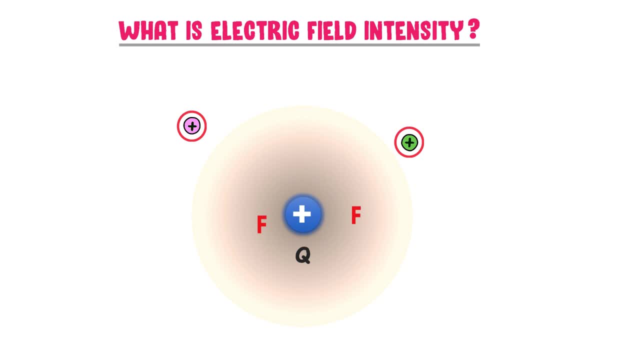 me repeat it: Positive test charge experiences force F inside electric field. We call this force as electric field intensity. Therefore, we define electric field intensity as the force F experienced by a unit positive charge Q, and the electric field is called electric field intensity. 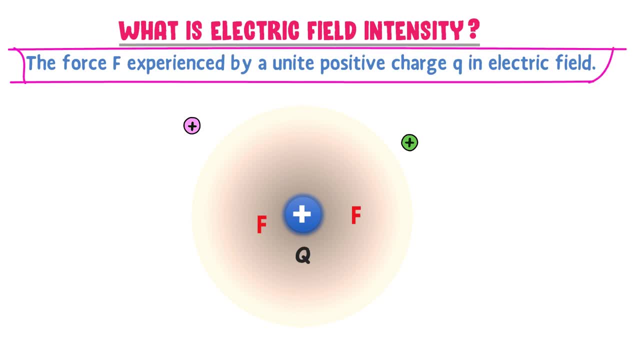 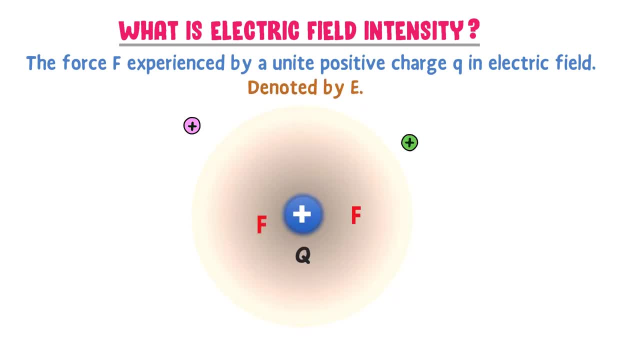 Electric field intensity is denoted by capital E. Electric field intensity is: E is equal to F upon Q, where E is the electric field intensity, F is the force and Q is the positive test charge. Note down that the SI unit of electric field intensity is Newton per coulomb. 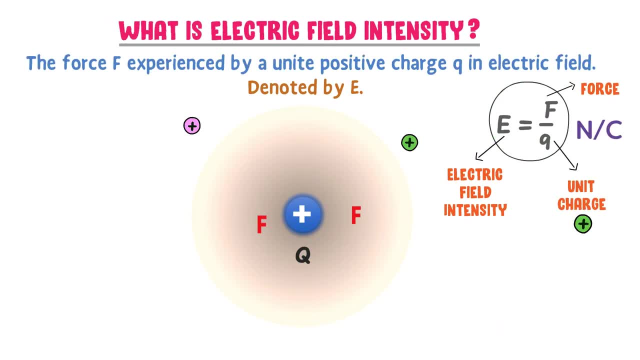 We know that force is a vector quantity. We know that force is a vector quantity seu electrici. So electrici is the vector quantity. So electrici is the vector quantity. field intensity is also a vector quantity. The direction of electric field intensity is the same. 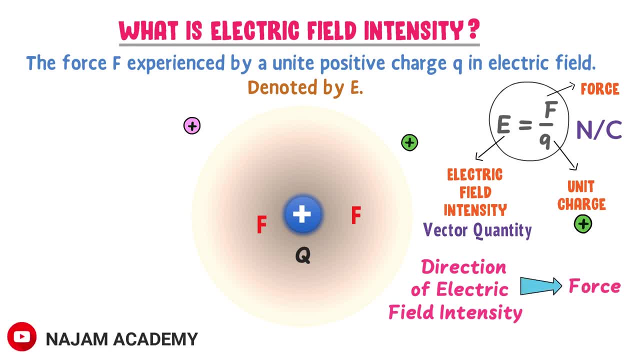 as the direction of force. For example, the direction of force on this test charge is like this: So it is also the direction of electric field intensity. Here. the direction of force on this test charge is like this: So it is also the direction of electric field intensity. 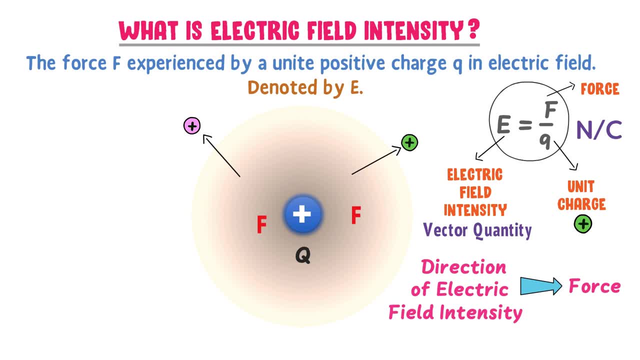 Now, as a bonus tip, let me teach you my favorite question: What is the difference between electric field and electric field intensity? Well, remember that electric field is the spherical region around any charged particle, while electric field intensity is the force of electric field exerted on a test charge or unit charge, Or we can also say that electric field 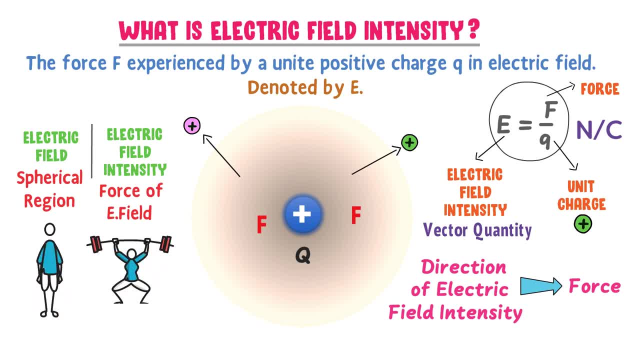 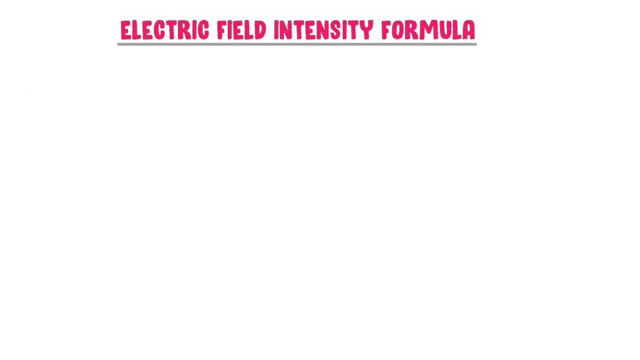 is the man and electric field intensity is its strength. Thus, remember that electric field is the region and electric field intensity is its force. Now let me derive the equation or formula of electric field intensity. Well, let's consider a big positive charge Q. We know that there is electric field around this charge. Now I bring a positive. 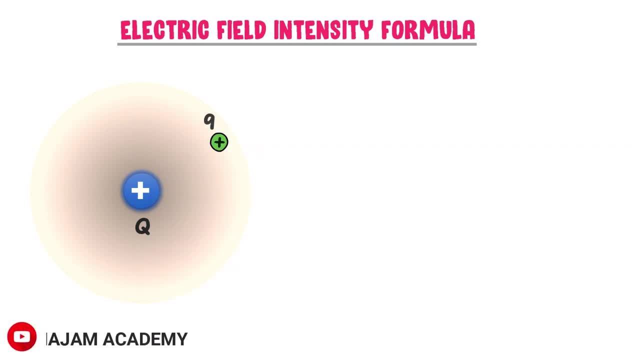 test charge Q inside the electric field of this charge. Let this test charge is present at a distance r from the center of this charge Q. We learned in the previous slide that this test charge experiences force F of the electric field. We know that electric field intensity is E is. 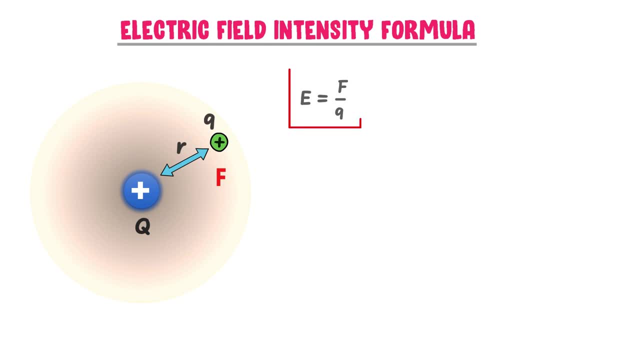 equal to F upon Q. Rearranging this equation, we write: F is equal to E into Q. Let I call this equation number 1.. Now, according to Coulomb's law, there is electrostatic force F between this test charge and this big power. 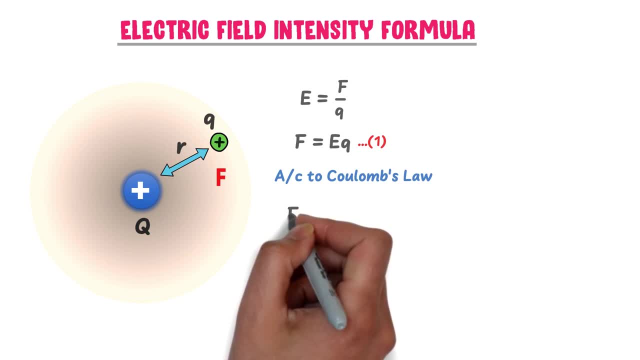 And this force F is equal to K, into the product of magnitude of the two charges upon the square of distance between them, Where K is the Coulomb's constant and its value is equal to 9 into 10, to the 9th Newton meter squared per Coulomb. Let I call this equation number 2.. Now plug in equation. 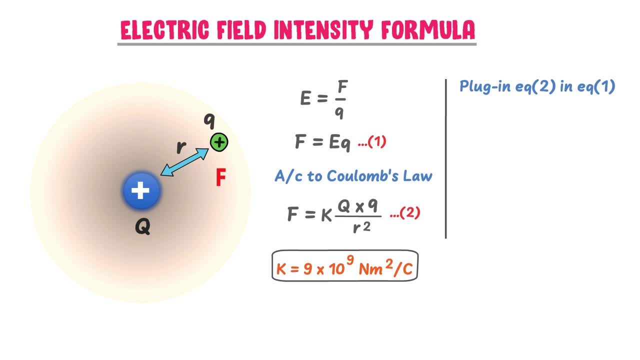 number 2 and equation number 2.. Now plug in equation number 2 and equation number 2.. Now plug in equation number 1.. We get E into Q is equal to K into Q, into Q upon r squared, This small Q and. 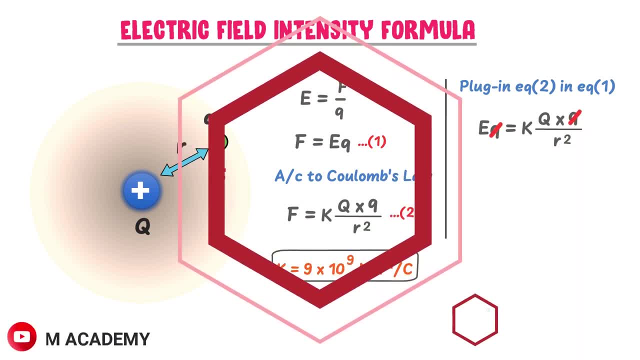 this small Q cancelled out on both sides, We get E is equal to K into Q upon r squared, Where E is electric field intensity, K is Coulomb's constant and Q is this charge and r is the distance from the charge. So electric intensity E is equal to K into Q upon r squared. Now note it down this: 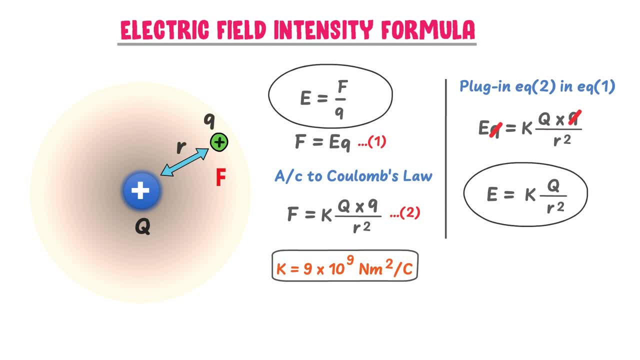 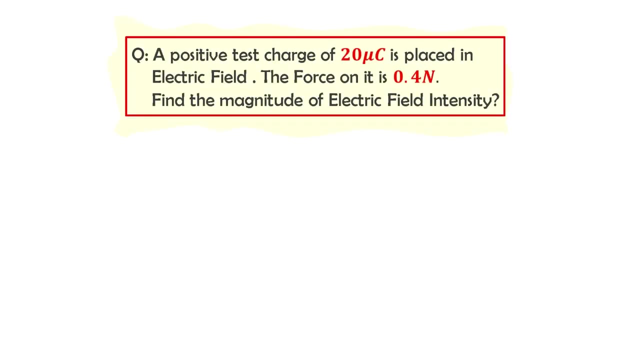 equation. and this equation I will show you how to crack any numerical of electric field intensity in any college exam easily. For example, consider that a positive test charge of 20 micro Coulomb is placed in an electric field. The force on it is 0.4 Newton. Find the magnitude of electric field intensity on a test charge. 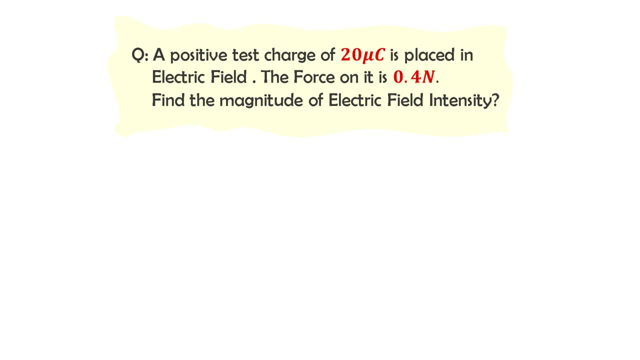 Well, firstly, let me draw a freehand diagram. Let consider a charge Q and its electric field. Let a test charge Q is equal to 20 micro Coulomb is present in this electric field. Let this Q charge exert force F. Force F is equal to 0.4 Newton on this test charge. We know that electric field intensity E is equal to F upon Q. 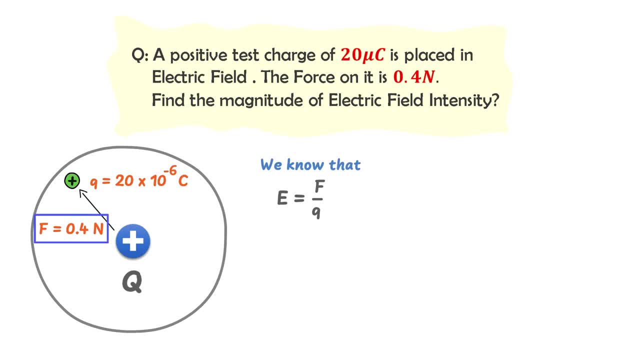 Here the force F is equal to 0.4 Newton on charge Q is equal to 20 micro Coulomb. So putting values in this equation, E is equal to zero point four Newton upon 20 micro Coulomb We get E is equal to 20,000 N per coulomb. 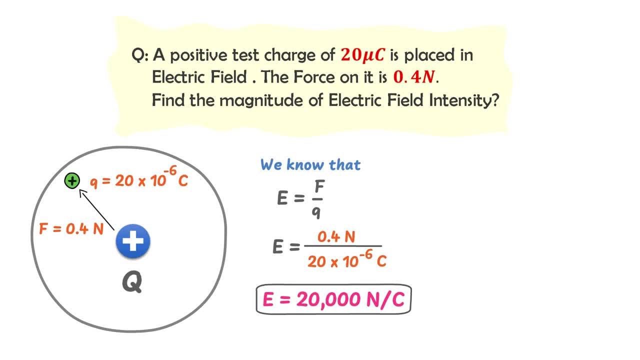 So the electric intensity of this charge Q on this test charge is 20,000 N per coulomb. I call such type of numericals as type 1 numericals Because we are given only the magnitude of a test charge and a force. 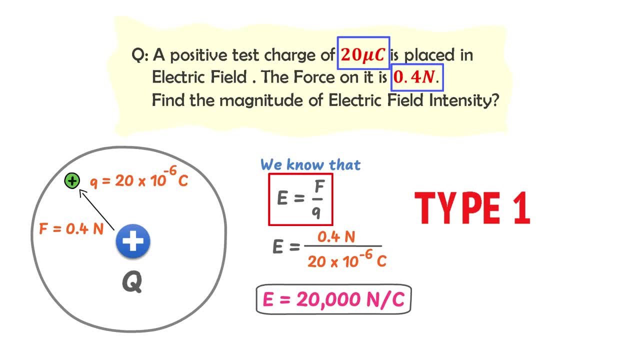 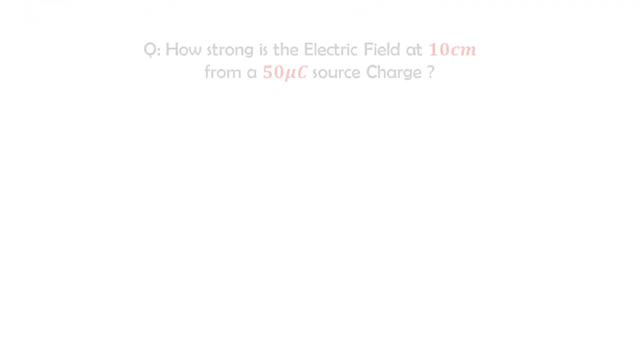 So we instantly use E is equal to F upon Q to get the required result. Therefore, remember the magnitude of a test charge and the magnitude of a force and type 1 form of numericals. Secondly, consider that how strong is the electric field at 10 cm from a 50 microcoulomb source charge? 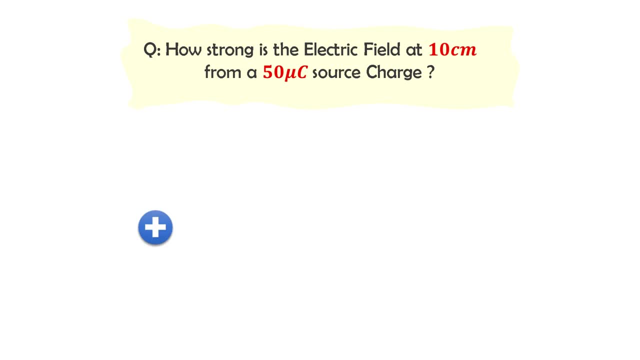 Well, let me draw a freehand diagram. Consider a point, Positive charge Q and electric field around it. Let the size of this charge is 50 microcoulomb. Now we are asked to find the electric field intensity at a point R is equal to 10 cm away from the center of this charge. 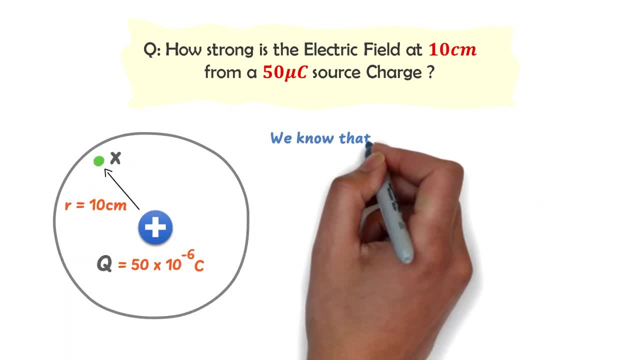 Let this point is X. We know that E is equal to K into Q upon R squared Here. K is the coulomb's constant and its value is equal to 9 into 10, to the 9th Newton meter squared per coulomb. 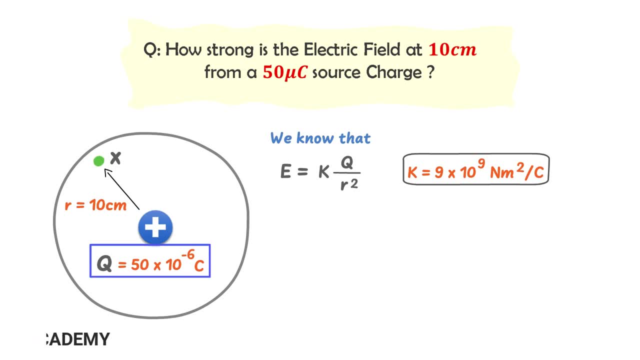 We know that Q is equal to 50 microcoulomb and R is equal to 10 cm, or R is equal to 0.1 meter. So plug in all these values in this equation. E is equal to 9.2.. 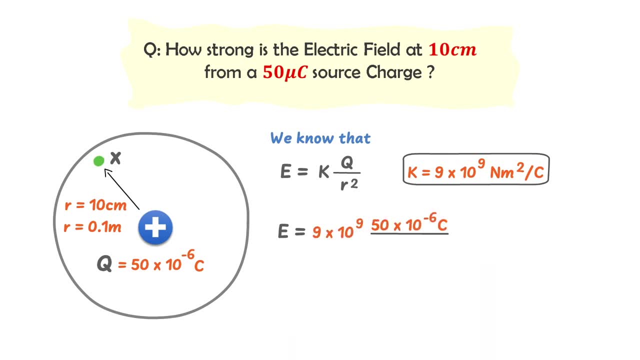 E is equal to 10 to the 9th and to 50 microcoulomb upon 0.1 squared I get 4.5 into 10 to the 7th Newton per coulomb. So the electric field strength or electric field intensity at 10 cm from the center of this charge is 4.5 into 10 to the 7th Newton per coulomb. 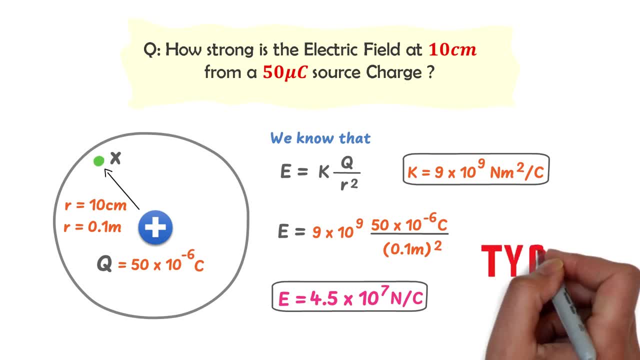 I call such type of Numericals as as type 2 numericals because no value of force or test charge is given. rather the magnitude or size of source charge is given and we are asked to find electric field strength at a certain distance. So remember that in type 2 form numericals magnitude of source charge and a point at a particular distance are given. 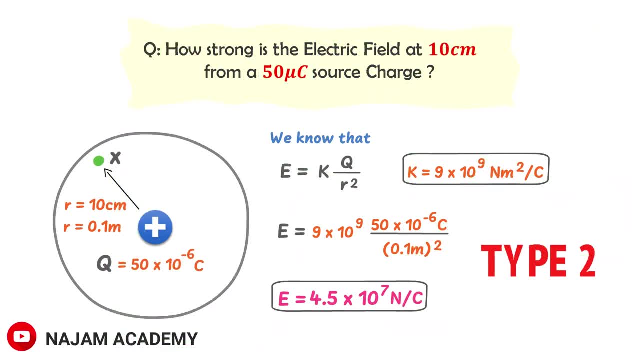 This was all About electric field and electric field intensity.